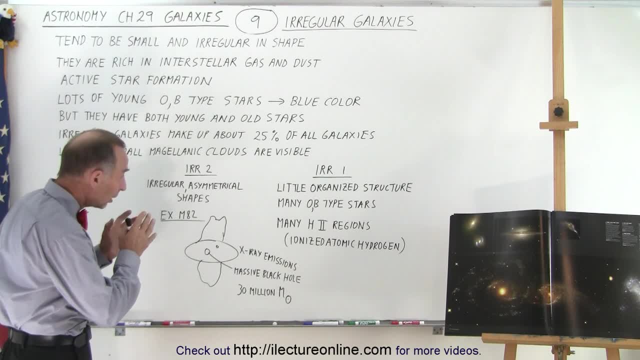 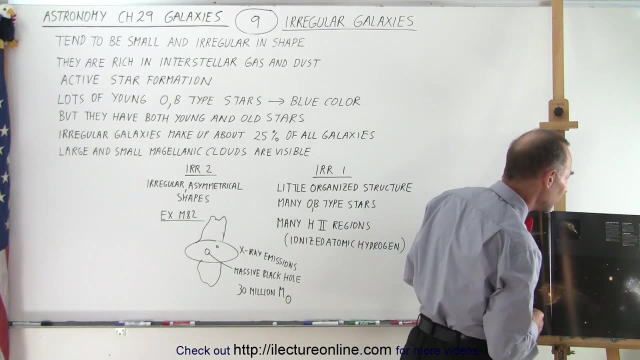 occur. So, as you can see, they tend to be small and they tend to be irregular in shape, And here we have a really nice little picture. Right here is the irregular galaxy. It's NGC 1427a. it's about 65 million years old. It's a really nice little galaxy. It's about 60 million years old. It's about 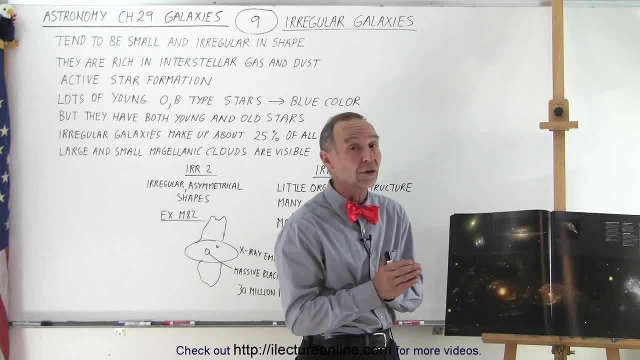 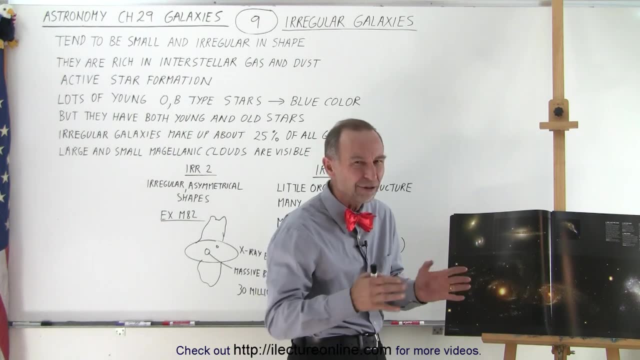 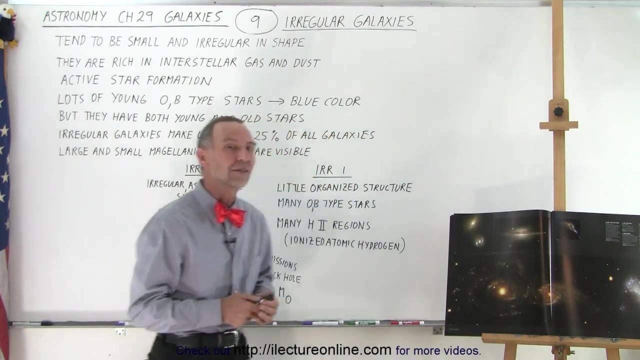 million light years from us and it's about 32,000 light years in length. now, that's actually quite large for an irregular galaxy. typically, irregular galaxies are like 5 to 10, 15 million light years across. this one is an unusually big one. now two of the famous irregular galaxies, of course, the large 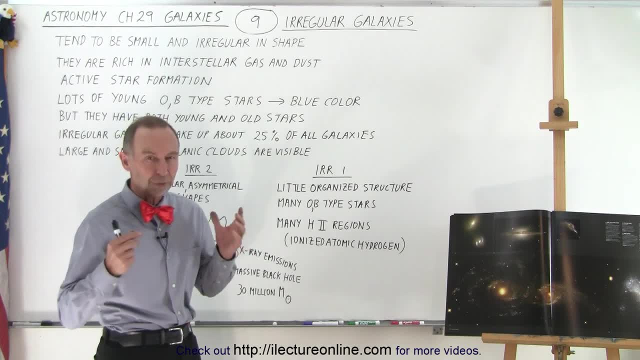 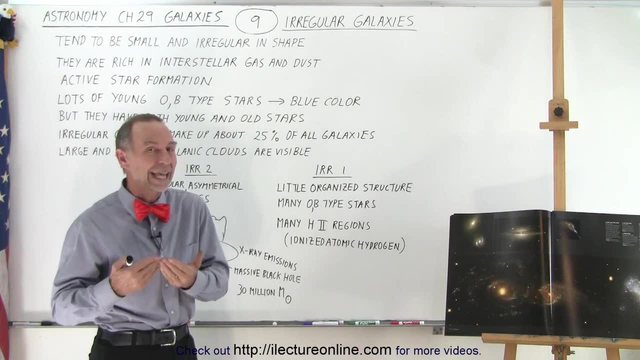 and the small Magellanic clouds, which are satellite galaxies of our own Milky Way galaxy, about 160- 170 thousand light years from us. so they're actually visible with the naked eye from the southern hemisphere. I personally have never seen them because I've never traveled to the southern hemisphere. but 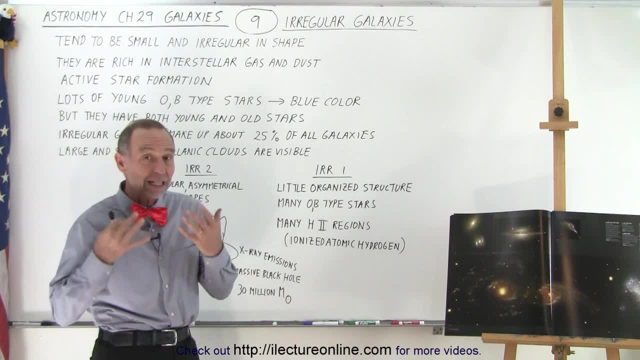 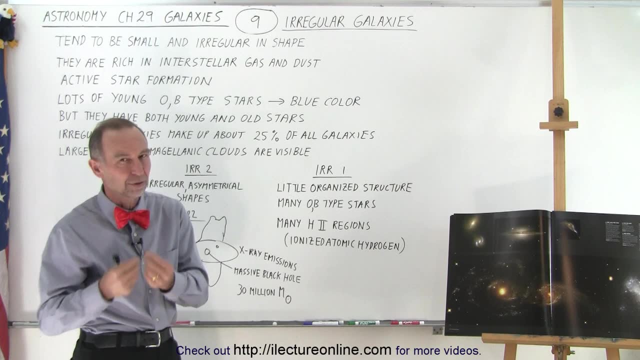 maybe one day I get the chance to do so, so that you can actually clearly see the galaxies in the sky. they look like fuzzy little patches and look like clouds. of course, with the naked eye you can't see the individual stars, they're simply too far away. but with a relatively small telescope you can actually see a little. 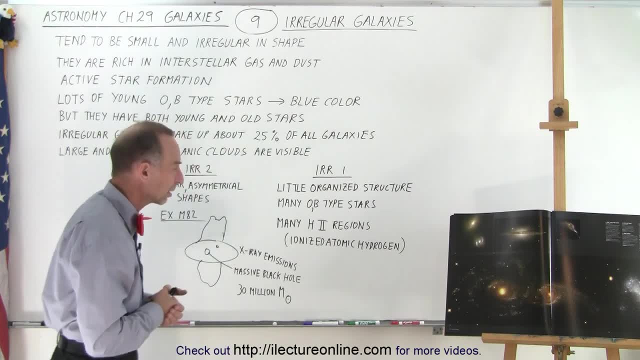 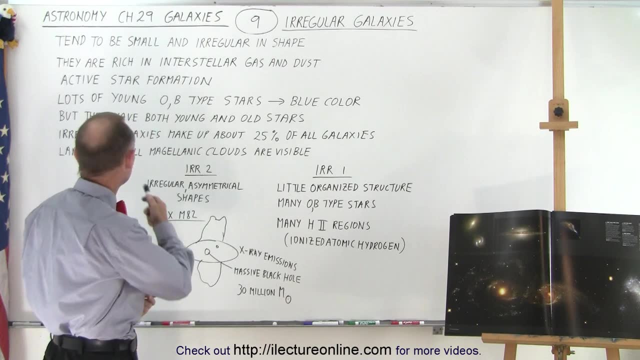 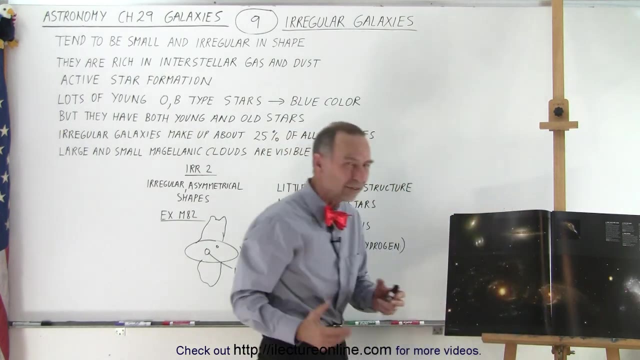 bit more detail in those small Magellanic and the small large Magellanic cloud. now they are rich, as we said, they're rich in interstellar gas and dust. so there's lots of star formation, active star formation, therefore a lot of young O and B type stars, and so, again, when you look at irregular galaxies, you tend to 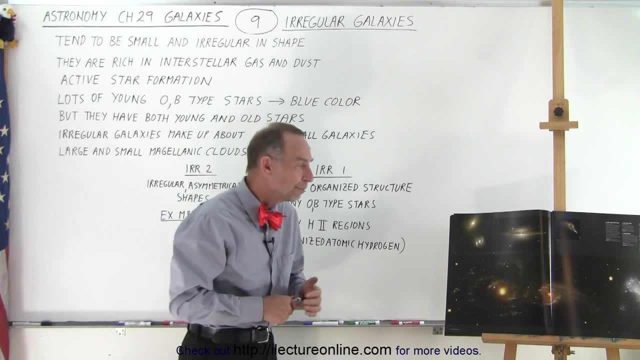 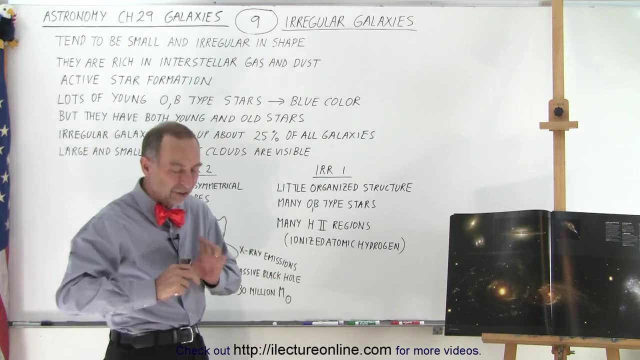 see the bluish color from the young, new, O and B type stars. they also have old stars, so they tend. there tends to be a mix and since there's no, not really a region where you have only the new stars and region where you have old stars, 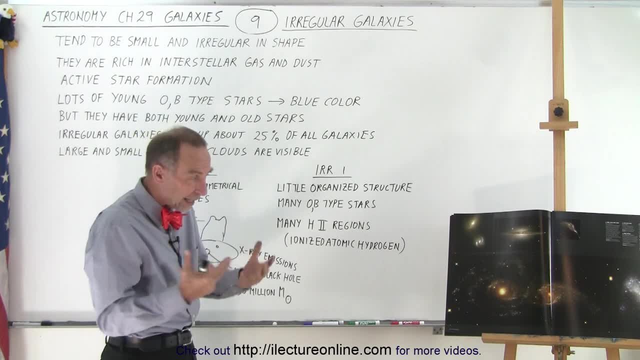 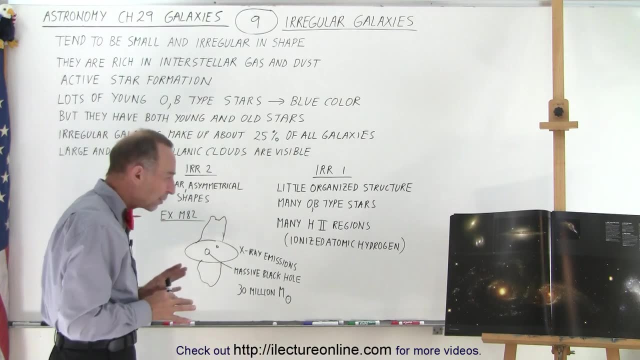 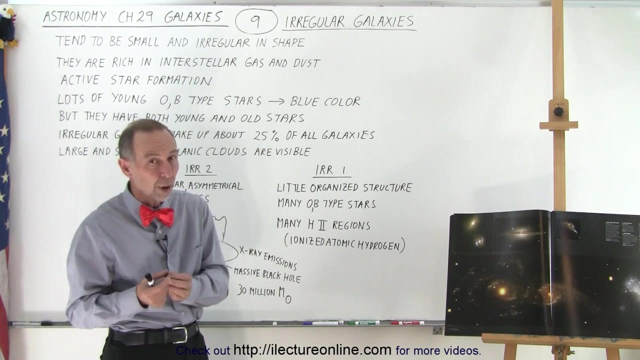 they're kind of intermingled so it's hard to see, but definitely intermingled. you have both the old stars and the new stars in irregular galaxies. irregular galaxies make up about 25% of all the galaxies in the universe. now that's hard to determine because, again, they're usually much smaller and much harder to. 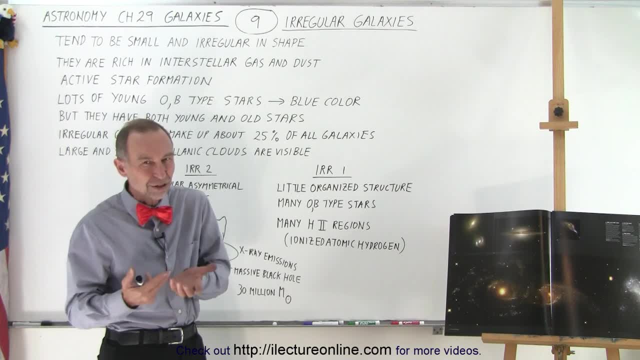 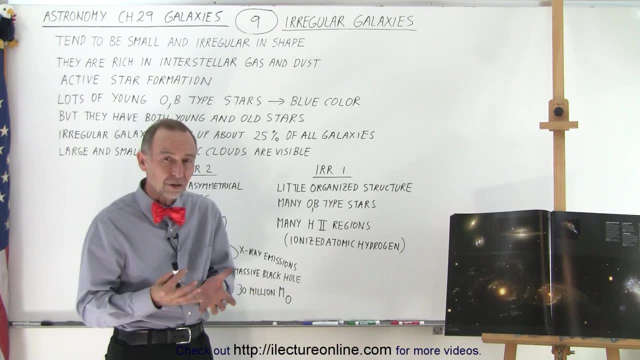 see the large ellipticals and the large spiral galaxies are much easier to see but they're quite abundant. in our own local group I think about 10 or 15 or so of the galaxies in our local group are the irregular type galaxies, so they're quite abundant relative. to the other galaxies in the universe. We divide the irregular galaxies into two groups. Again, there's a subdivision in the irregular galaxies, so we call them IRR1 and IRR2.. The IRR1 are the more typical irregular galaxies. There's little organized structure, it's just. 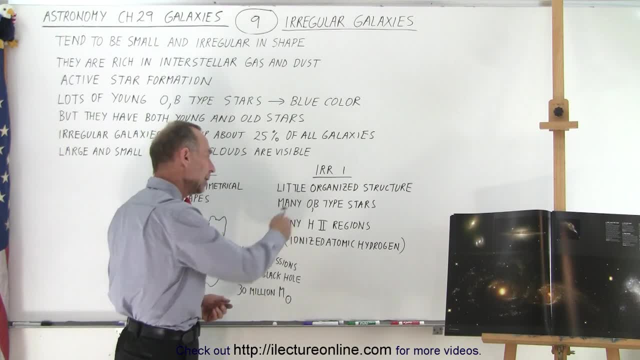 basically a blob of stars, Again many O and B type stars, so lots of star formation taking place, and you'll find that there's many, and I think many should have two N's in it, doesn't it? Many One N, Really, It looks strange, Hmm, Okay, well, all right, I've 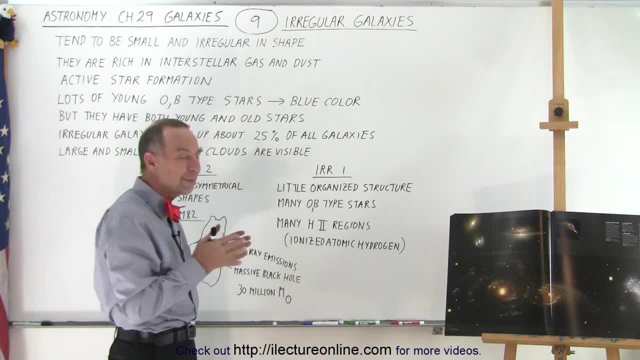 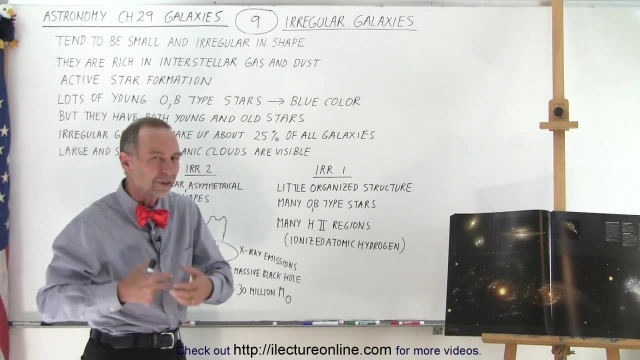 been corrected. many is indeed one N, And so there's many what we call H2 regions. Now, H stands for hydrogen and 2 indicates that it's ionized, So there's a lot of atomic ionized hydrogen. ionized because there are a lot of O and B. 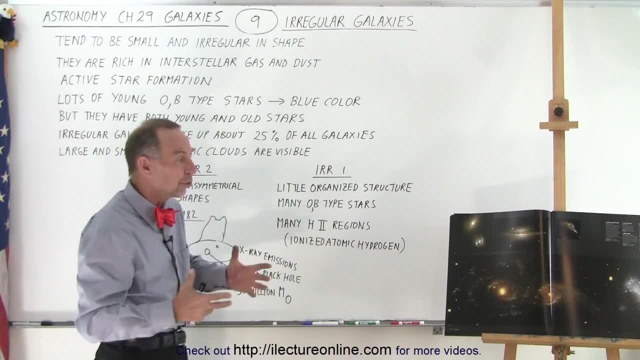 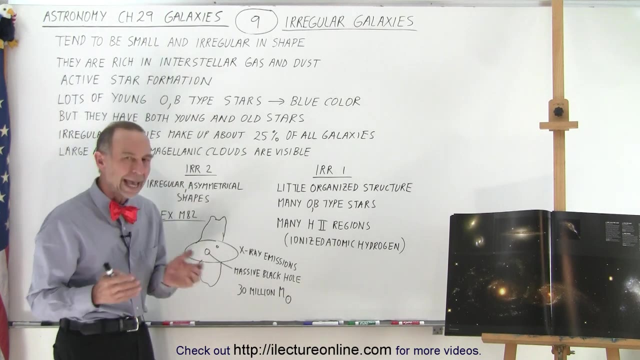 type stars. so there's a lot of UV radiation inside those galaxies, therefore ionizing the gas regions into what we call H2 regions. So that's very typical for IRR1, irregular one type galaxies. The irregular twos is a special category. What's special about them? 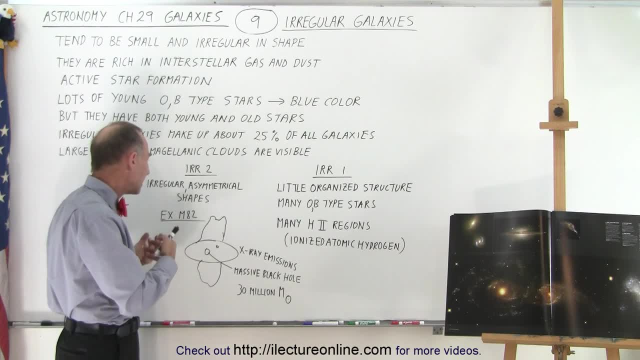 is that they tend to have a symmetrical, irregular type shape. There's so many different types of galaxies. There's something going on in these galaxies that's unusual. So, for example, M82 is one of those irregular galaxies that are kind of out of the ordinary because at 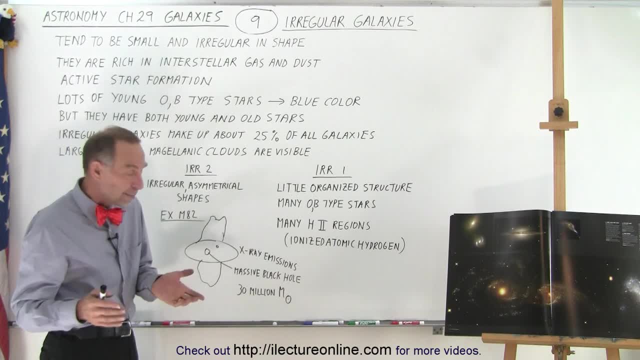 the very center there's a massive black hole with an equivalent mass of 30 million suns, so it's a huge black hole. Then there's a smaller black hole not too far away from the center, which has about a mass of about 500 solar masses, and we see a lot of X-ray emissions. 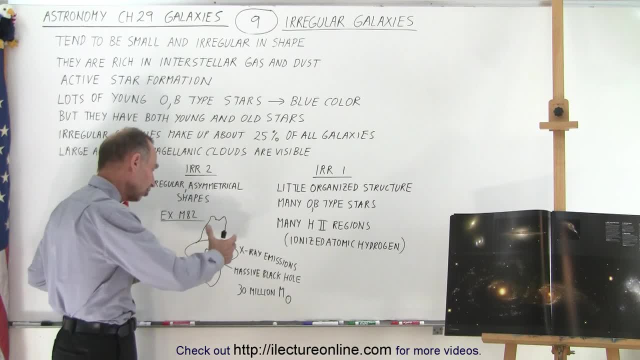 and whenever there's a lot of X-ray emissions, there's a lot of energy, It can push and shove into the galaxy out of shape, and so you see that there's these different structures caused by the high intensity radiation and the influence of a massive black hole at the center.